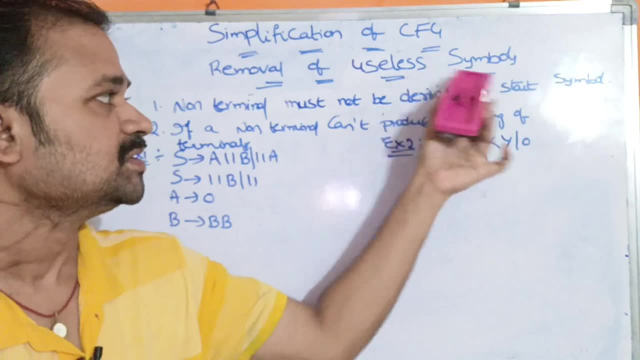 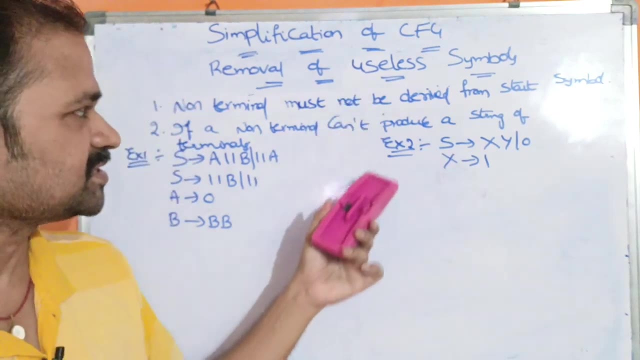 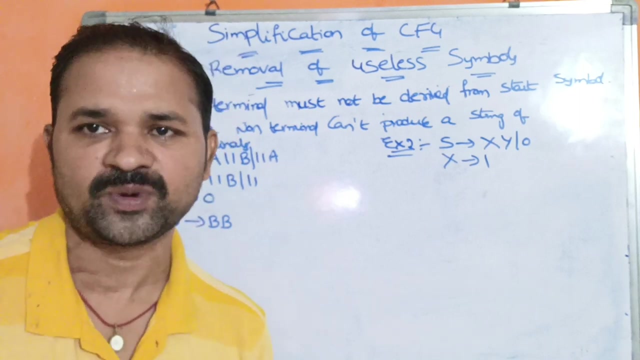 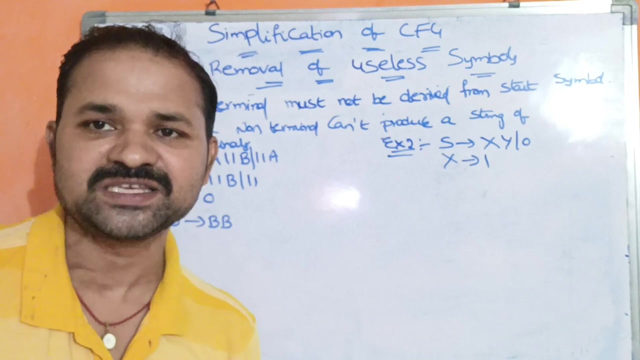 Here our target is: we want to remove useless non-terminals, useless uppercase letters. So here we have two steps, are there? We can call a symbol as a useless symbol if it satisfies two properties. The first property is non-terminal, must not be derived from the starting symbol. 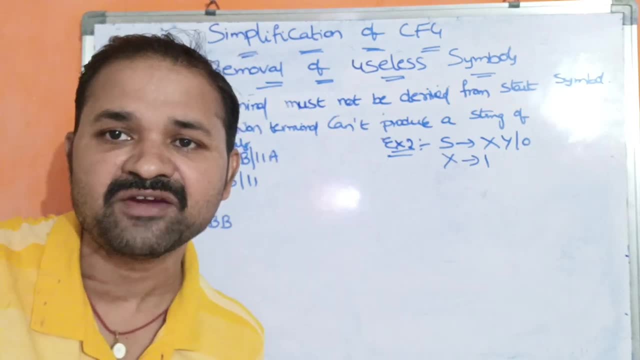 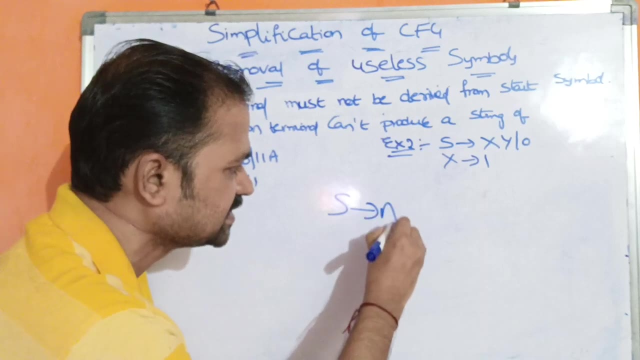 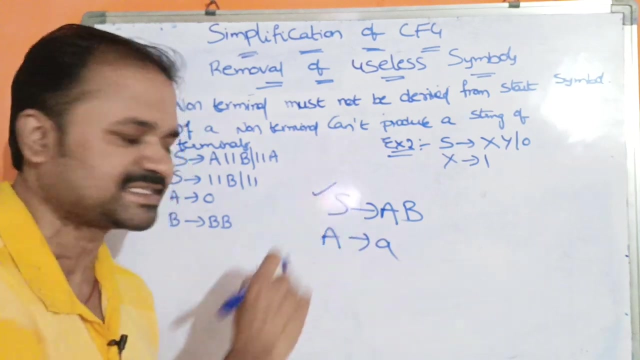 So if a non-terminal is not derived from starting symbol, then we can call that symbol as useless symbol. Let we have a production like this: S produces AB, A produces A. Here the start symbol is S. Why? Because start symbol means. 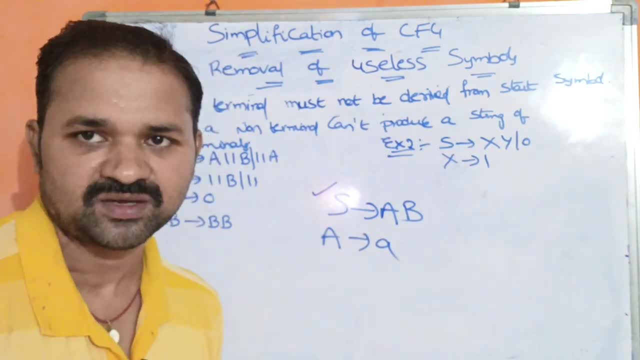 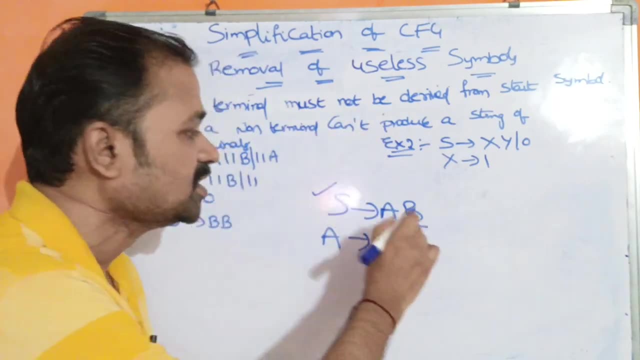 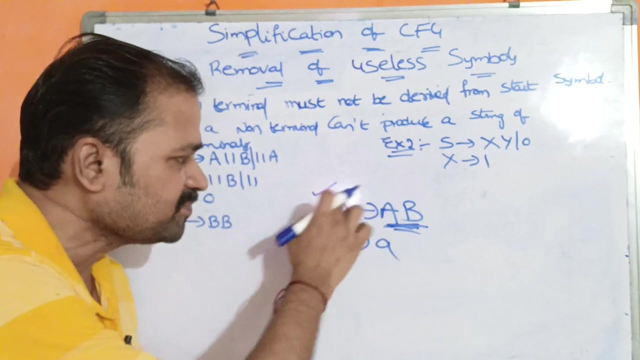 the first two production left hand side, non-terminal. So here the non-terminals must be derived from the start. Non-terminals must not be derived from the start symbol. Here, if you take A, A is derived from the. here we have A production, A produces A, But B productions are. 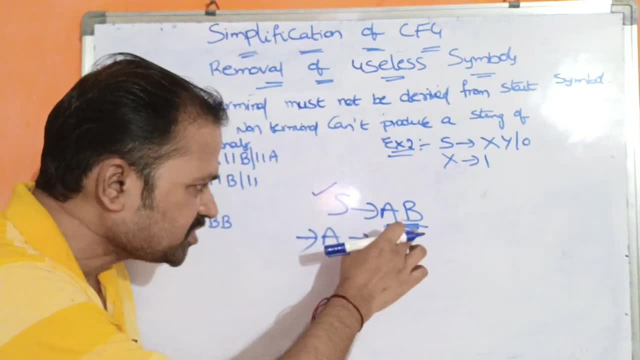 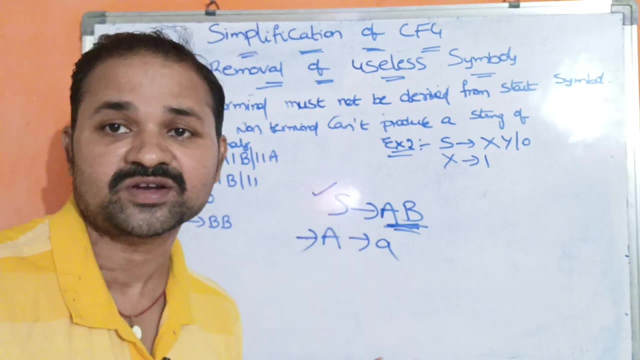 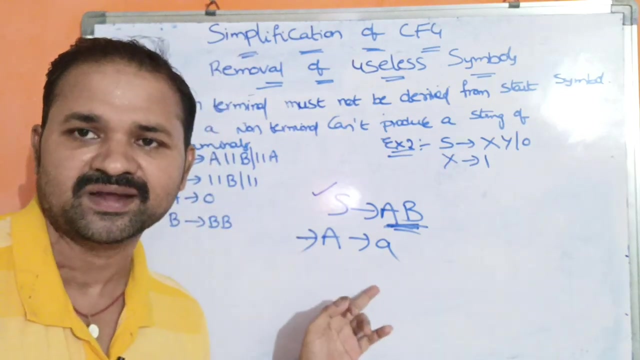 not there. Okay, Here B productions. B productions are not there in this problem. So we can say that B is not derived from the start symbol. So we can say that B is useless symbol. Why? Because B productions are not available here. B is not reachable from S, Whereas A is. 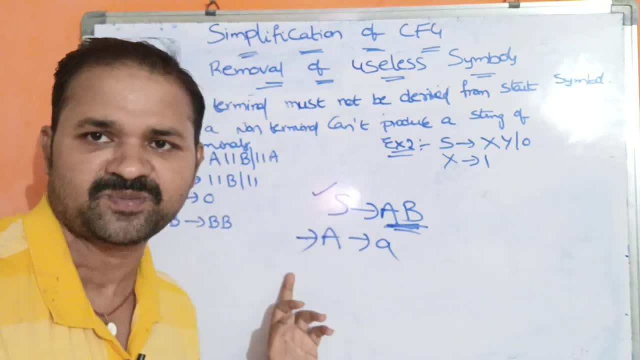 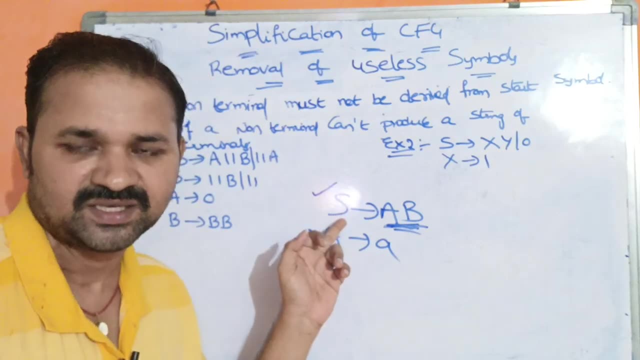 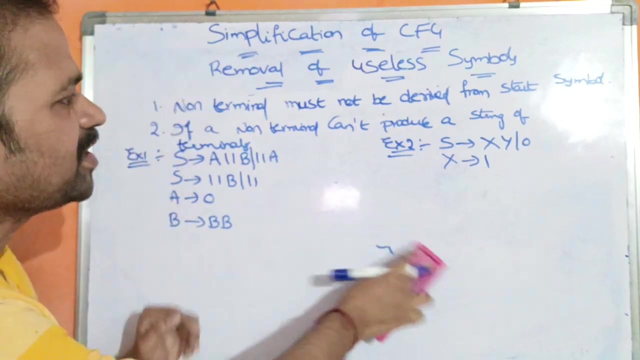 A is reachable from S. Why? Because A productions are present in the problem, But B productions are not present in the problem. So we can say that B is not reachable from S. So that's why we can say that B is useless symbol. Okay, And the second condition is, if a non-terminal 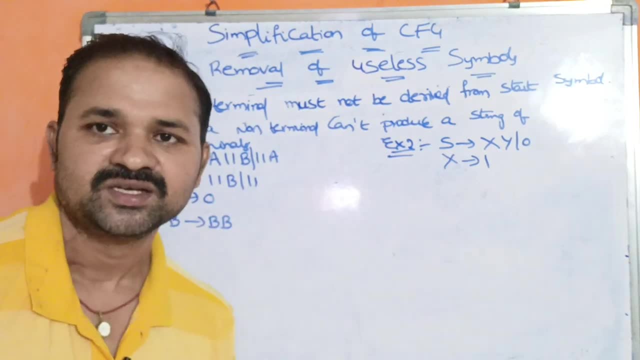 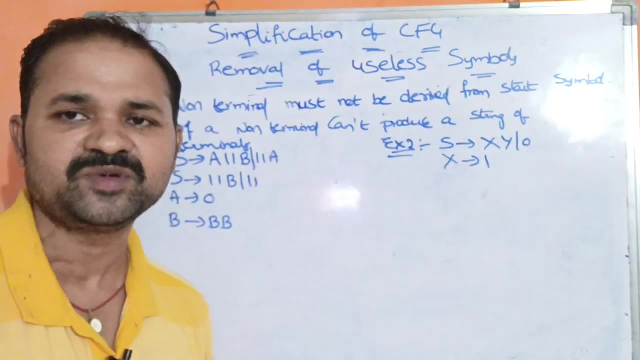 cannot produce a string of terminals. So every non-terminal must produce a string of terminals. If a non-terminal cannot produce a string of terminals, then we can say that, we can say that it is useless symbol. So totally, we have two properties, are there? 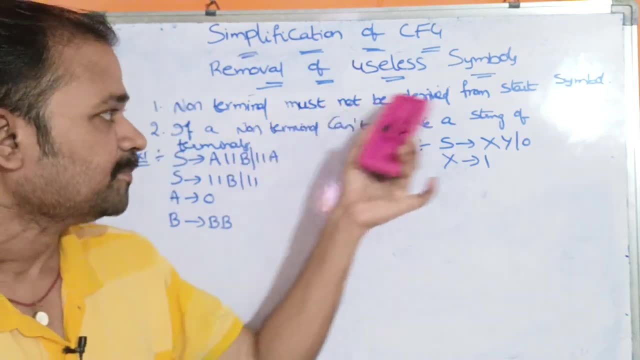 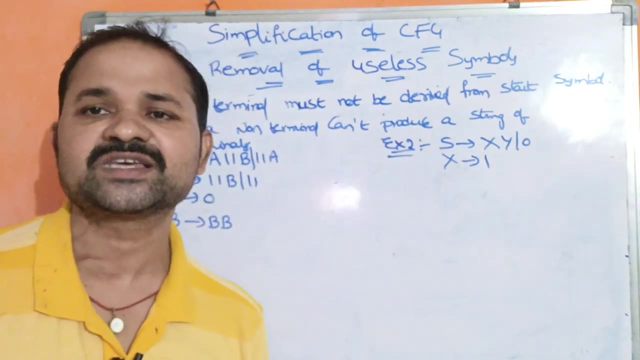 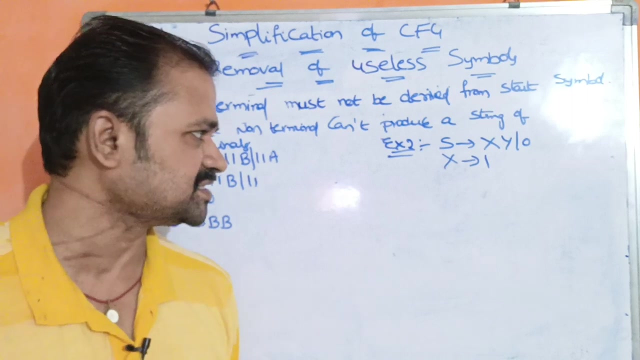 What is the first property? Every non-terminal must not be derived from the start symbol. And the second property is: if a non-terminal cannot produce a string of terminals. Let us solve these two examples. Let us see the second example first. This is the simple example. 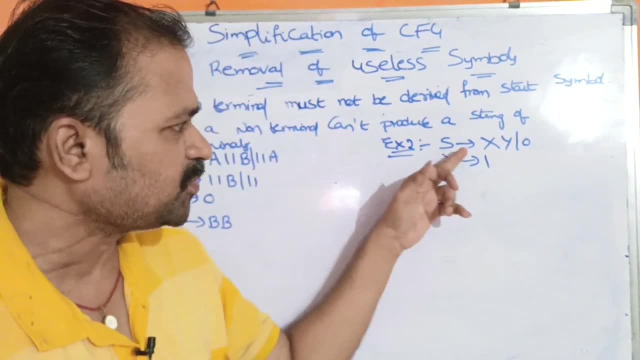 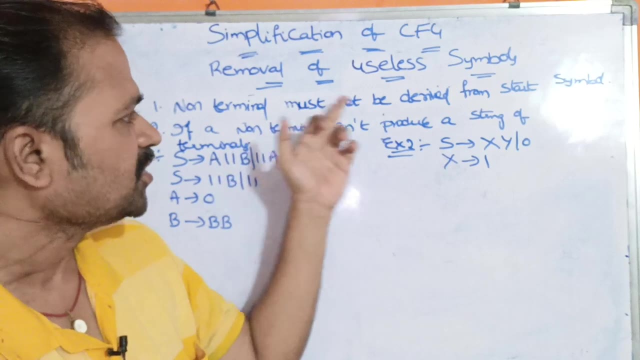 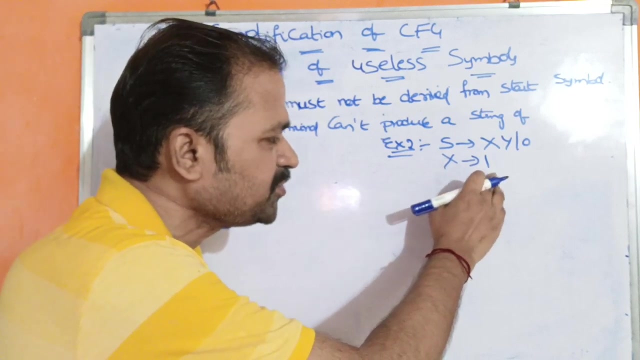 So here we have two productions are there? S produces x, y are 0, x produce 1.. Here what is the first condition? Non-terminal must not be derived from the start symbol. If you take this problem, here we have x produces y, x implies y, So we can say that x is reachable. 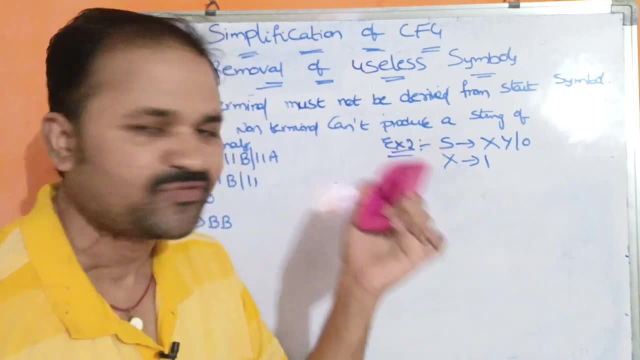 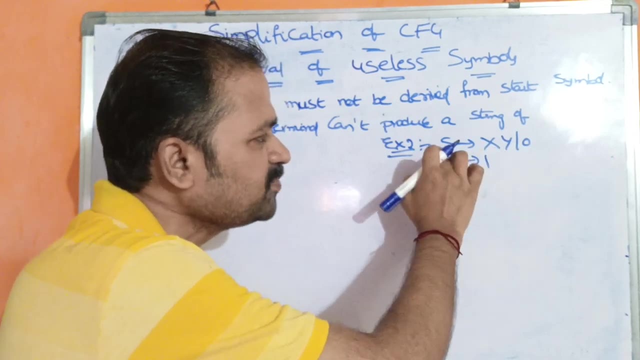 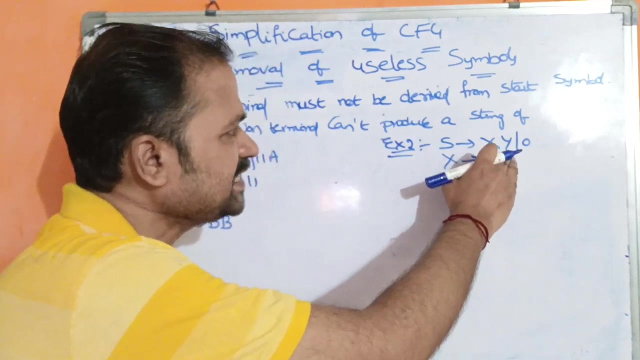 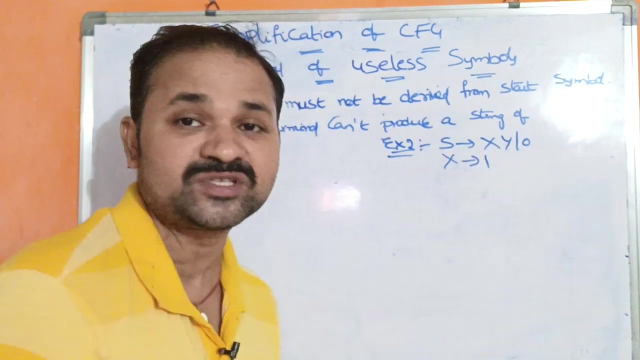 from S. We can reach to x from S, But y productions are not there in the problem. So we can say that y is not reachable from S. So this non-terminal is not derived from the starting symbol. So we can say that x, y is useless production. Why? Because here. 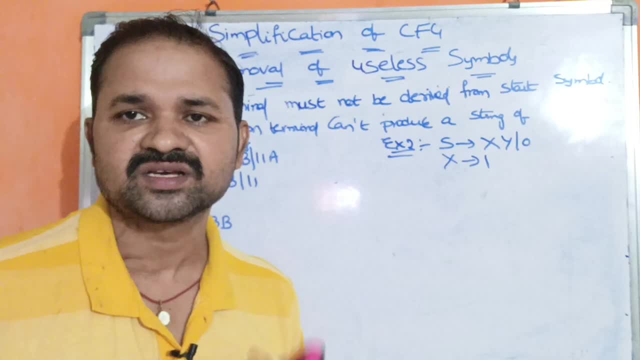 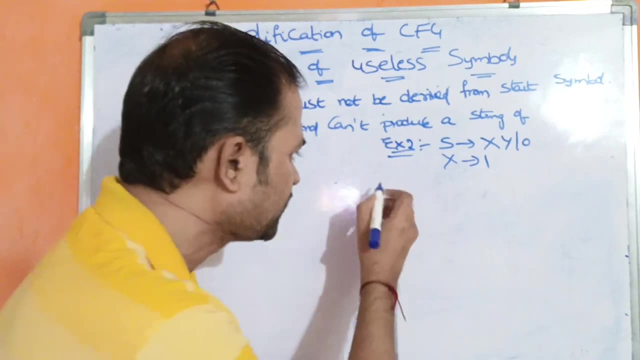 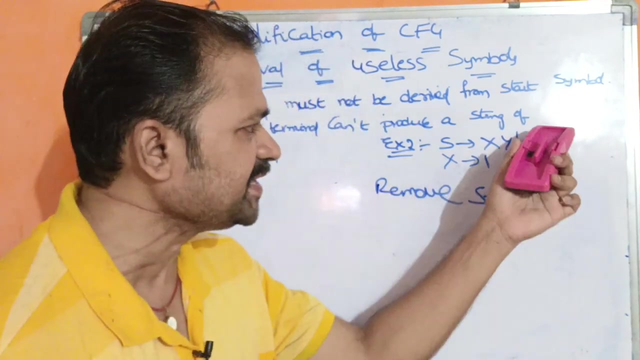 y is useless symbol, So all the productions associated with y are useless. But in this problem we have only one production, that is x- y, So we can remove. S implies x, y. And what is the next one? S implies 0.. Here every non-terminal. 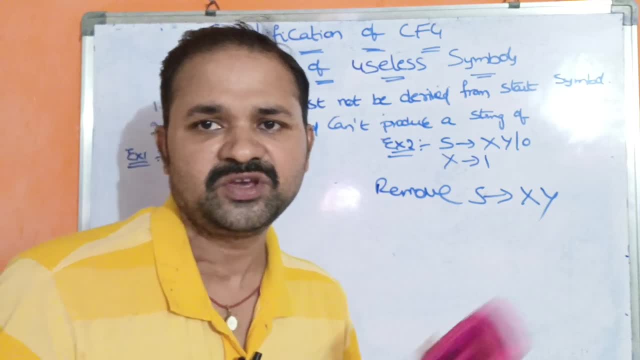 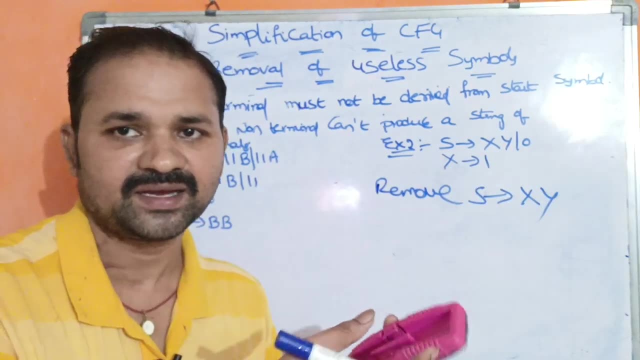 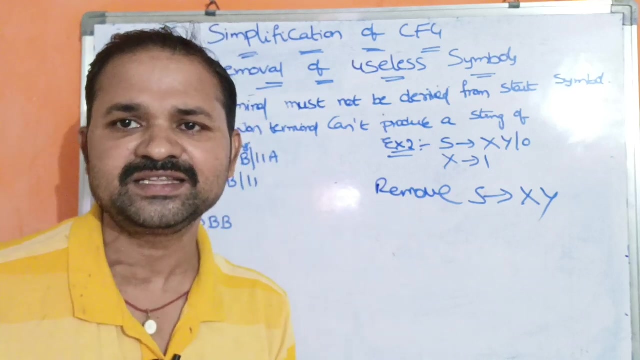 must produce a string of terminals. So if your non-terminal produce a string of terminals, then there is no problem. OK, That is, that is useful, symbol only OK. But if your non-terminal cannot produce a string of terminals, then we can say that that is useless. OK, So we. 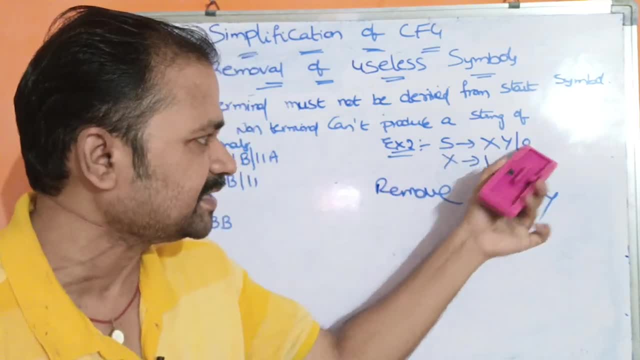 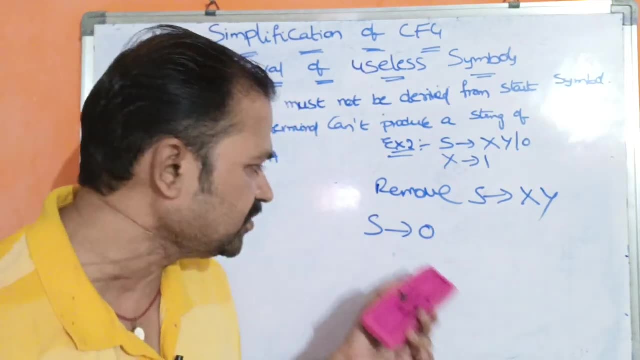 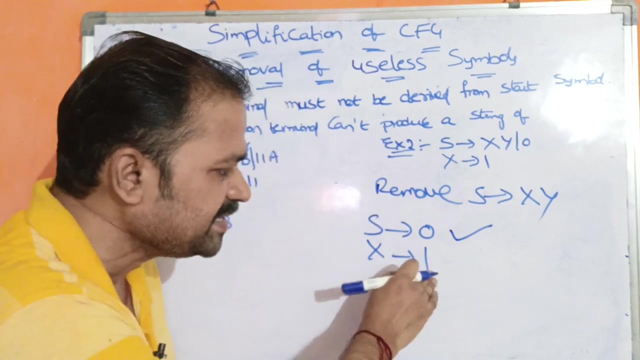 less symbol. Here this non-terminal is producing s produces 0.. This non-terminal is producing terminal. 0 is nothing but terminal only. So it is producing terminal symbol. So this is useful production. Next x implies 1.. So this non-terminal is also producing terminal symbol. So this is. 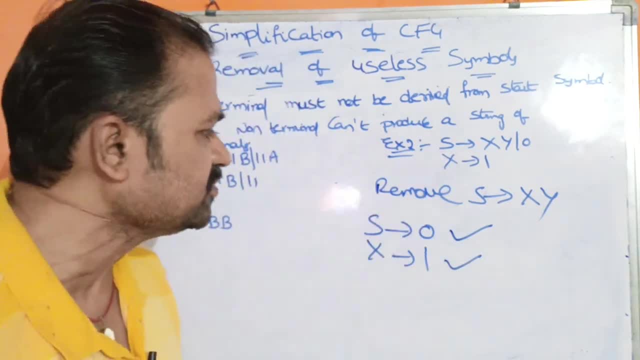 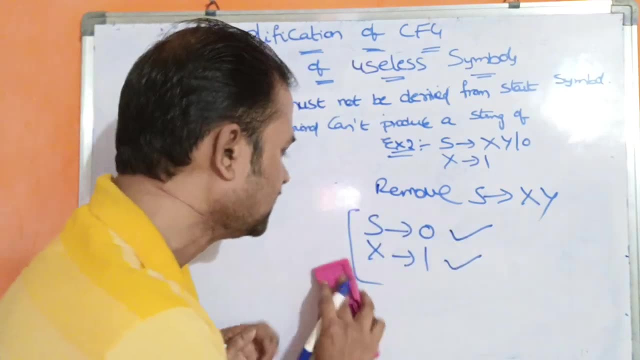 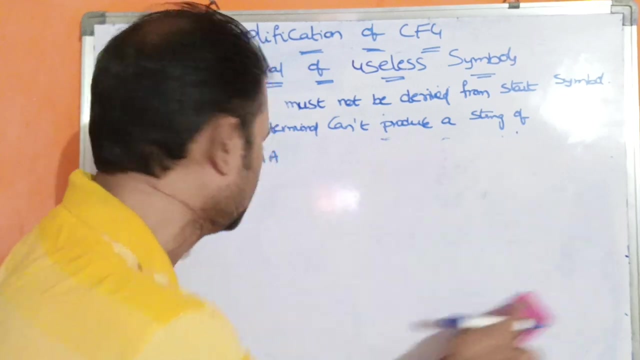 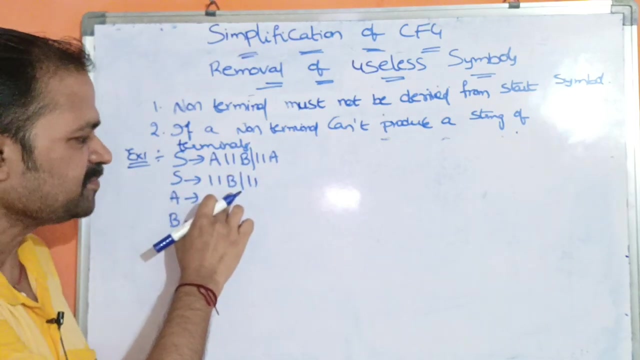 also useful productions. So here, after eliminating useful symbols, the grammar is these two productions: s implies 0, x implies 1.. Let us solve the second first example so that you will get the perfect clarity If you have any doubts. s produces a, 1, 1, b or 1, 1, a s produces 1,. 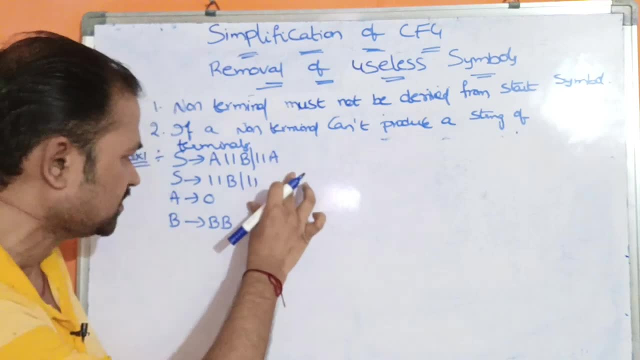 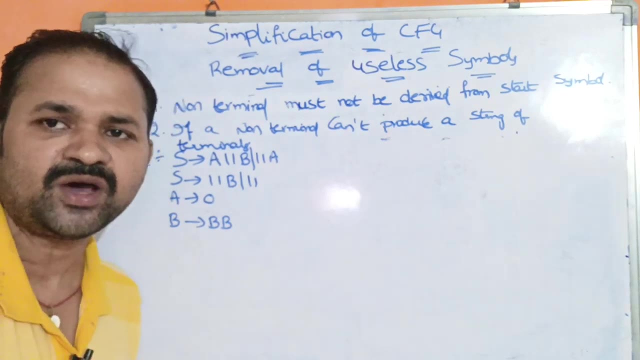 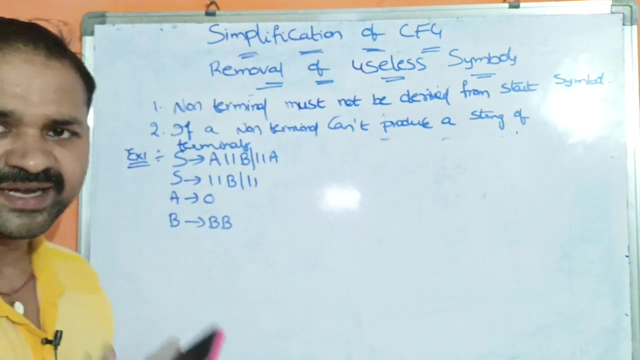 1, b or 1, 1.. So totally we have four productions associated with s. Next, a produces 0, b produces b, b. So now our target is we have to remove useless symbols from the grammar and we need to write the final grammar. Let us see: 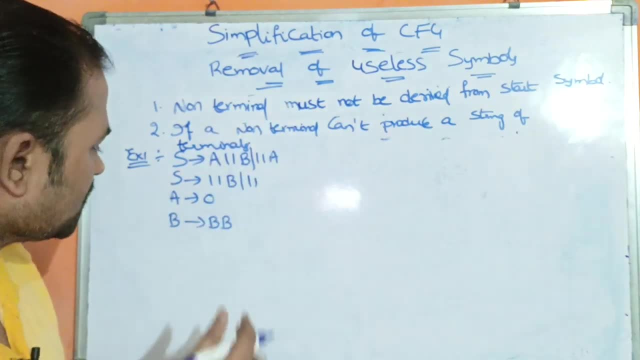 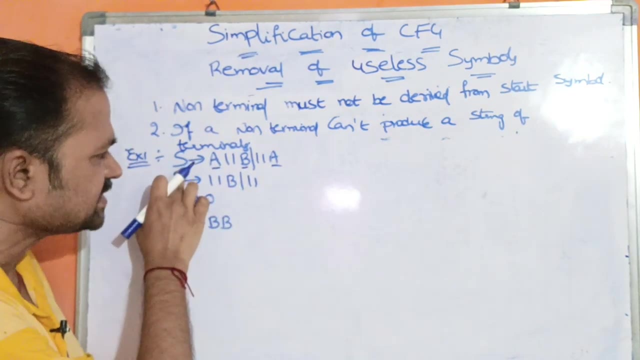 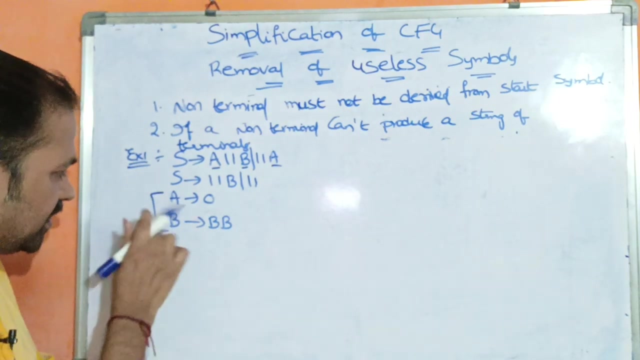 the problem here? What is the first point here? First, let us check the non-terminals. Here we have a, b, Here we have a. So here s is producing two non-terminals, a and b. Let us check whether a and b are there or not. Here we have a production as well as b production, So we can say that a is. 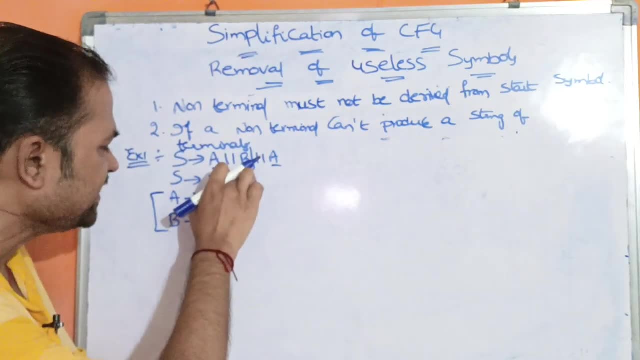 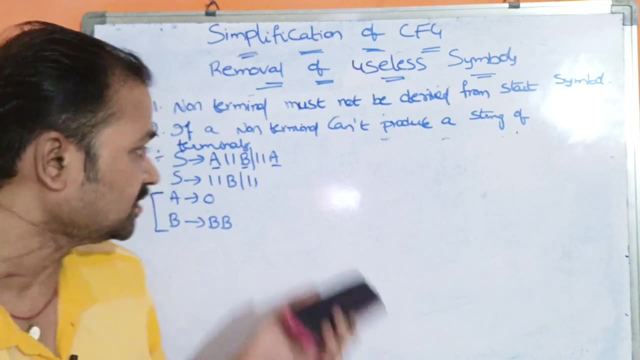 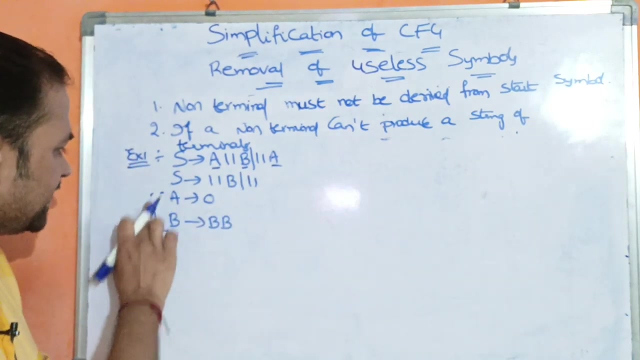 reachable from s, as well as b is reachable from s. So a and b are useful productions only. A and b are not. they are not useless symbols. A and b are useful only, So there is no need to remove these two. Next, let us see the second condition. What is the second condition If a non-terminal cannot? 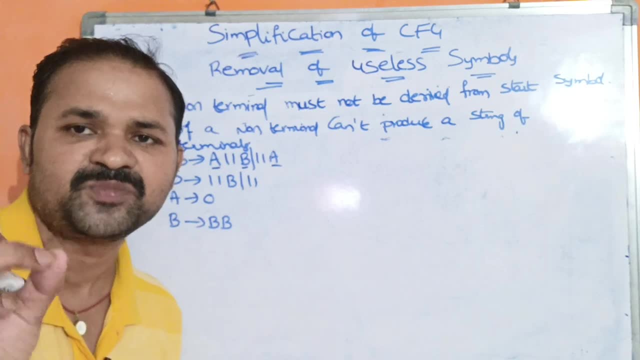 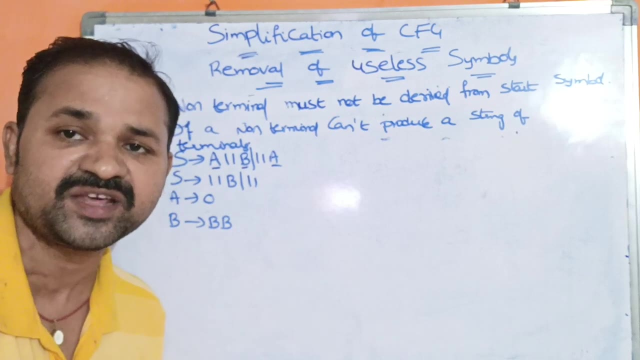 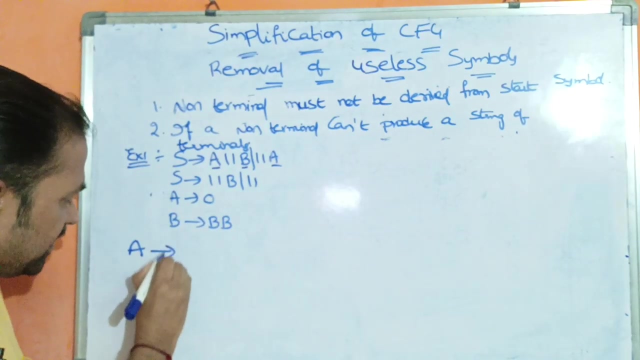 produce a string of terminals. So if a non-terminal produce a string of terminals, then that is useful, Whereas if a non-terminal cannot produce a string of terminals, that is useless. Okay, Let us start from the a. Let us consider a. a. What are a productions? a produces 0.. a implies 0.. So this: 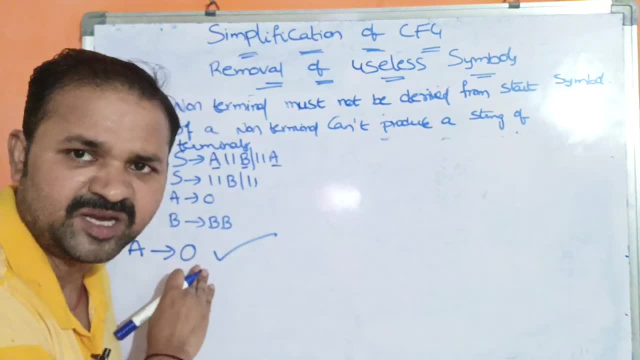 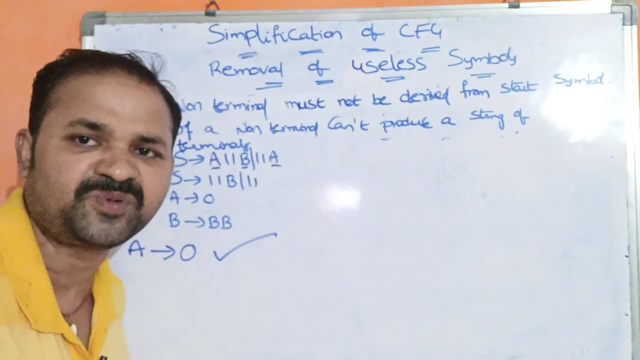 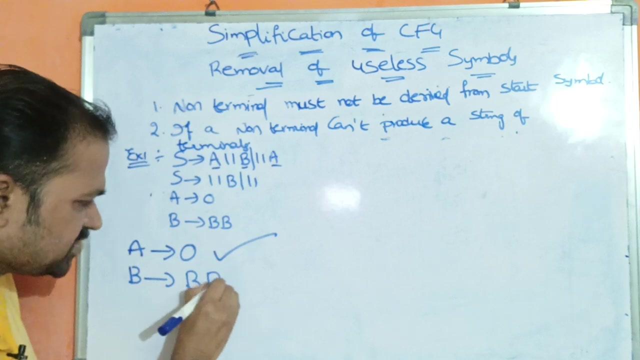 is useful, production only. Why? Because this non-terminal is producing terminal symbol. This is useful only. There is no need to remove this one. Okay, If it is useless production, then we have to remove that one. Next production: b implies bb. Let us check whether it produces terminals or not. So what is b here? b produces. 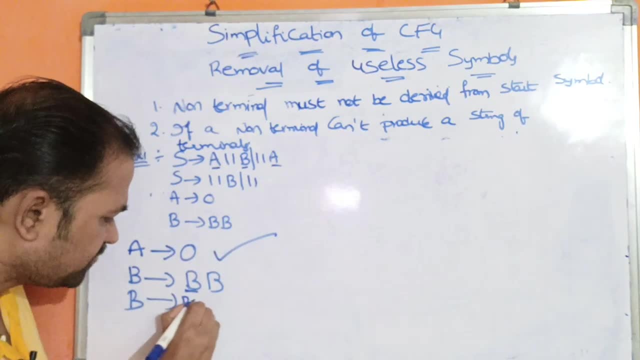 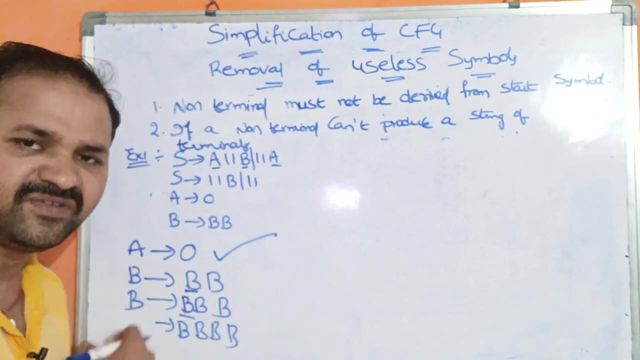 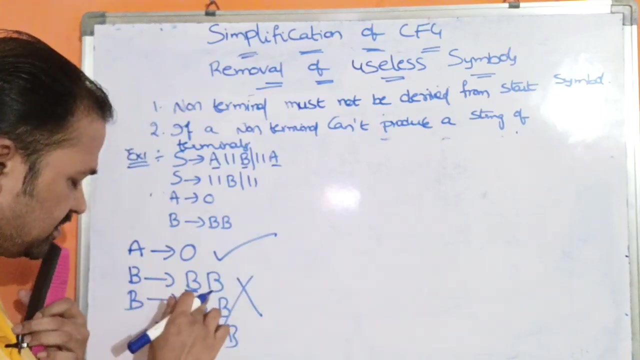 only bb. So in place of b we can substitute bb. Next again, in place of b we can substitute bb. So likewise we will get n number of bs while doing the derivation. So we can say that this is what Useless production, This is useless production. So here b is useless production. 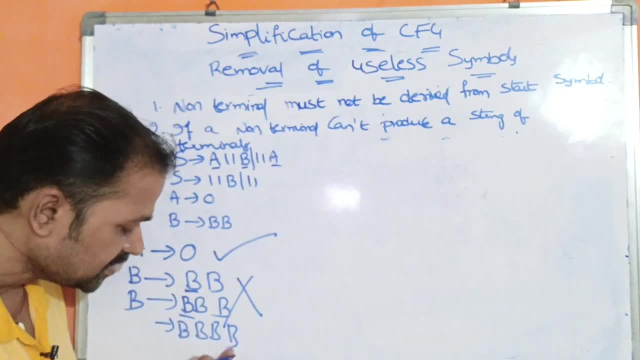 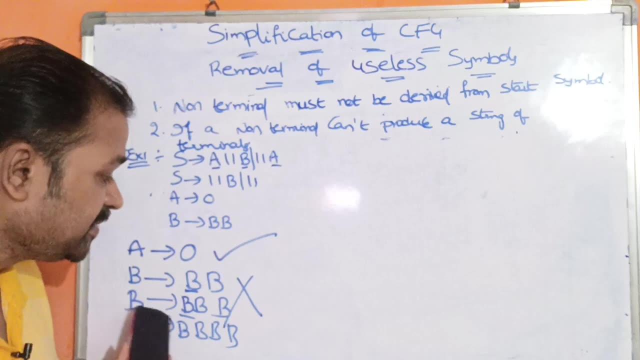 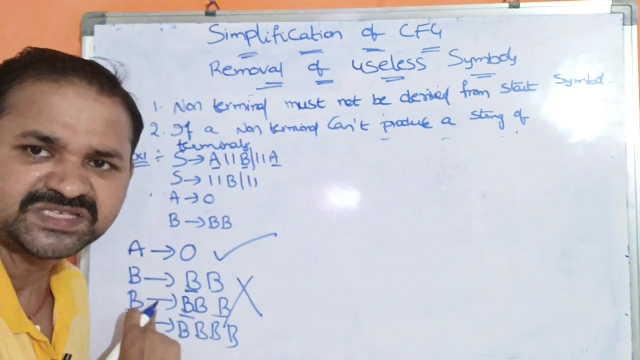 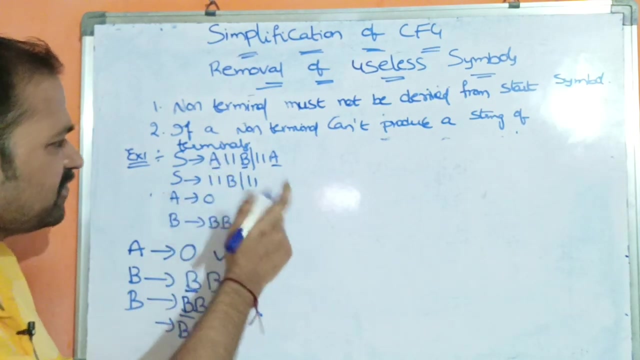 Why? Because b is not producing terminal symbols, So we can say that all the productions associated with b are useless. Why? Because b is what A useless non-terminal. So what are the productions associated with b? Here we have a11b, So s produces a11b. Here we have b. 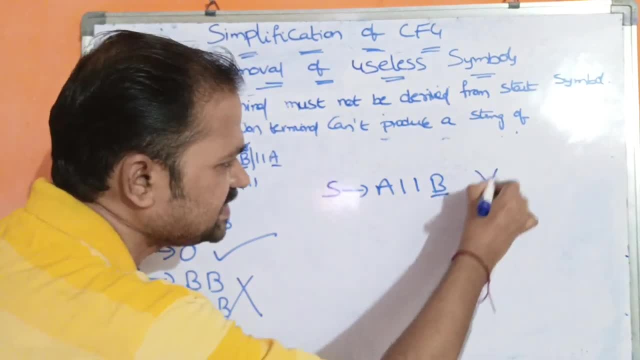 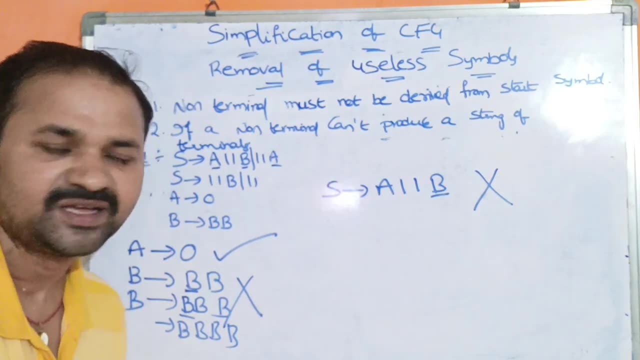 This production is associated with b, So we can say that this is useless production. Why? Because b produces only non-terminals. b doesn't produce terminals. If it is not producing terminals, then we can say that it is an useless production. So this is useless one. Next s produces a11b. 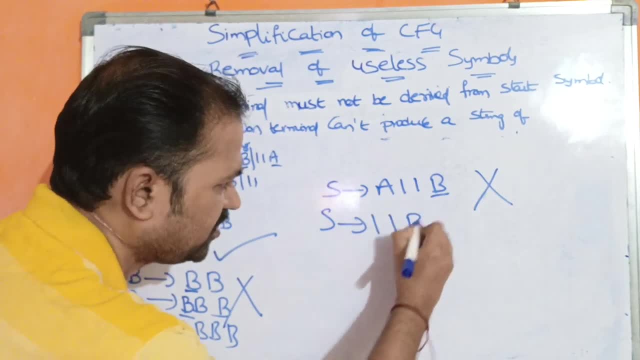 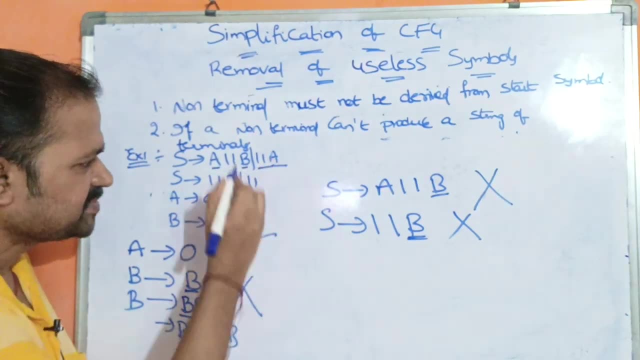 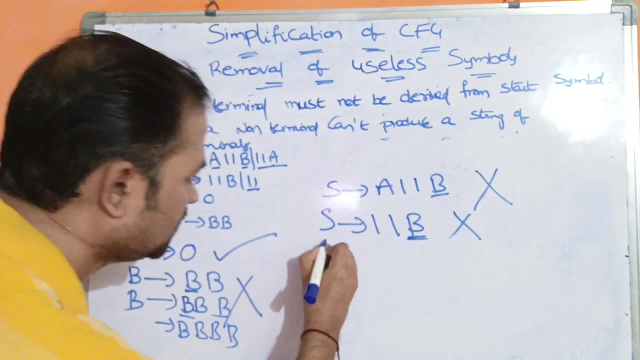 So this is also useless production. Why? Because this production is associated with b. Next, what are the remaining productions? Here we have one production s produces a11a. Here we have another production s produces a11.. Let us check whether those two are useful or useless. s produces a11a. s produces a11.. What 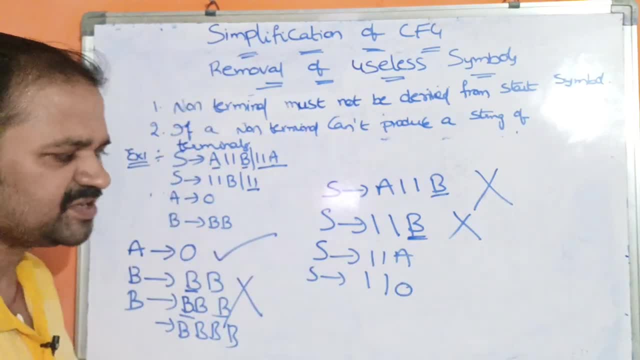 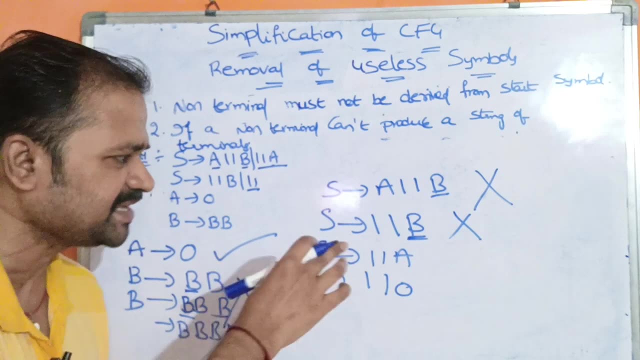 is a, a means 0. So here s is producing a110.. So it is nothing but terminals. Terminals are nothing but digits. only Terminals are digits, lowercase letters and some symbols: Plus, minus, star, left, parenthesis, right, parenthesis likewise. 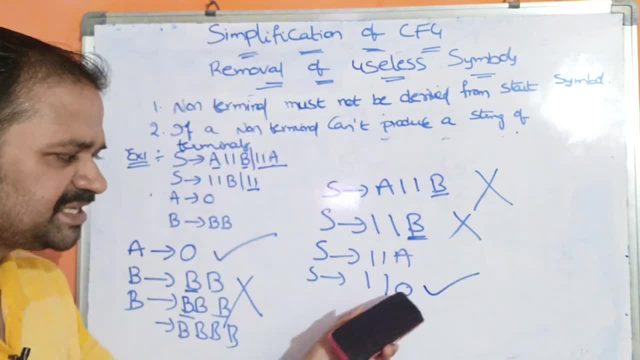 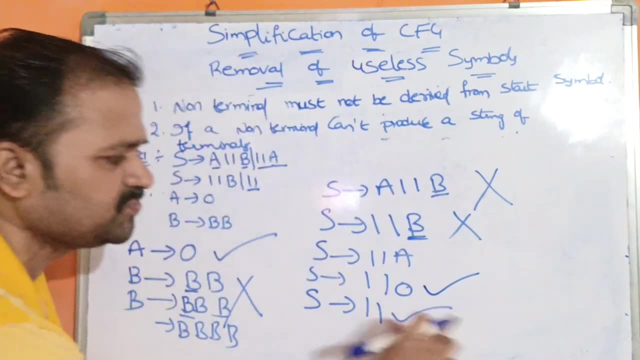 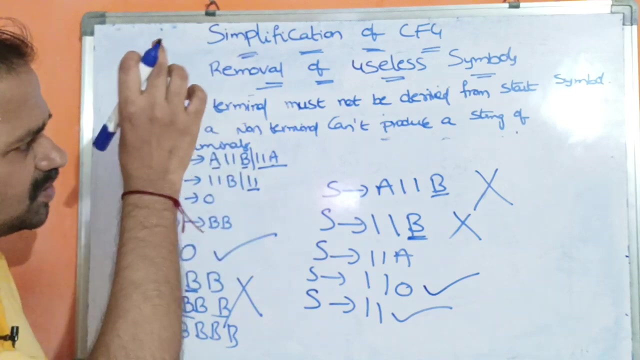 So this is useful? only Why? Because it is producing terminals. Next one s produces a11.. s produces a11.. So this is also useful production. Why? Because it is producing terminals. So what are the? what are the? what is the grammar after eliminating useless? 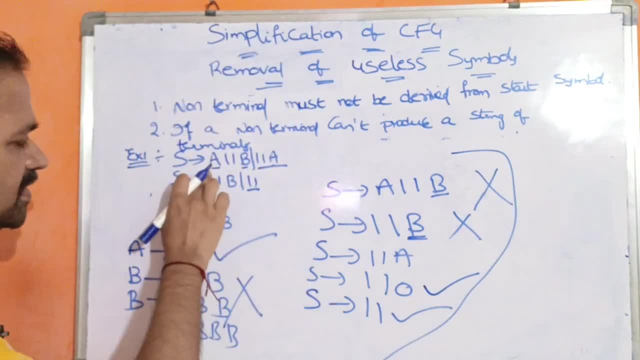 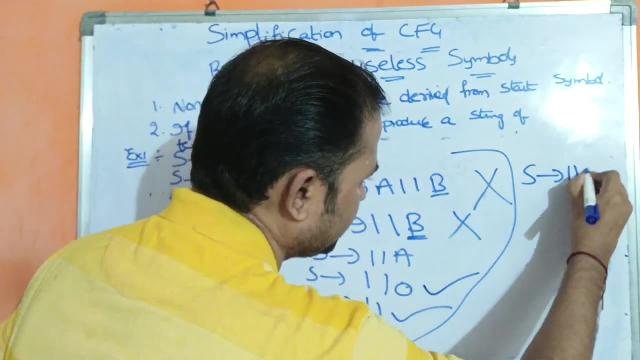 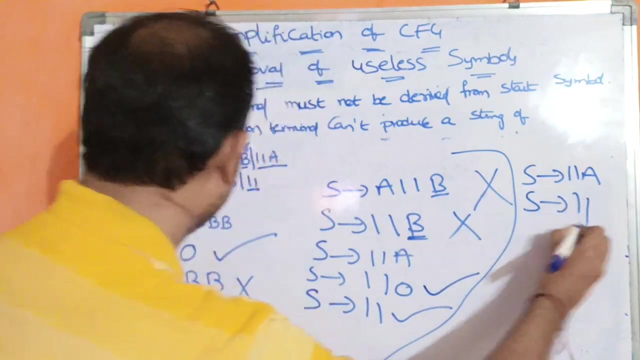 symbols. The final grammar is here. Here we have eliminated a11b. Next s produces a11a, So this is useful only. Next 11b is useless. s produces 11.. Next a produces 0. So after.